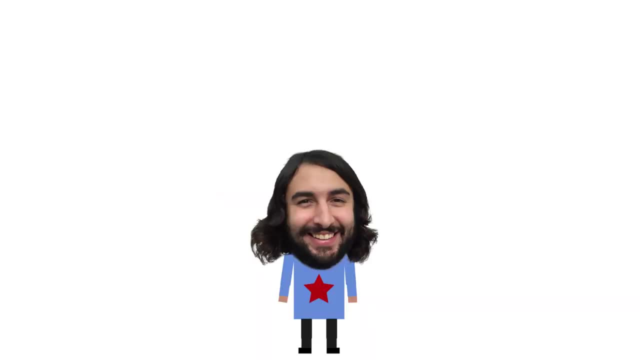 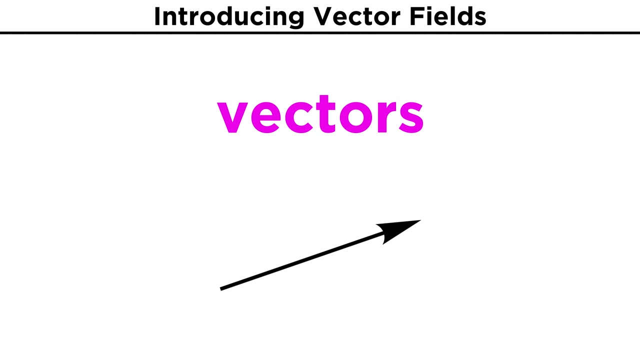 Professor Dave, again let's check out vector fields. We spent a lot of time with vectors when we learned about linear algebra and, not surprisingly, we won't be done with them any time soon. We are used to vectors being made of components which are scalars. 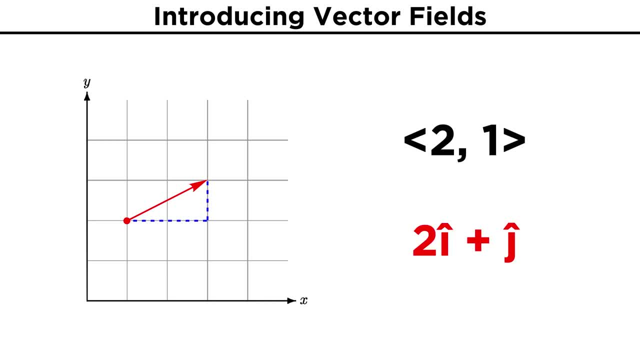 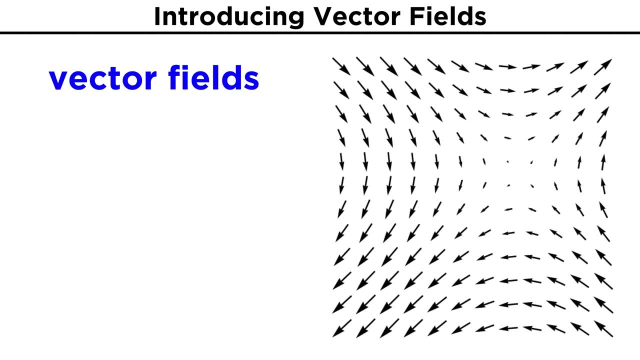 For example two, one which can also be written as two i plus one j. We then got used to being able to move these vectors around however we wanted, but now we are going to introduce vector fields, which can be thought of as functions that take in. 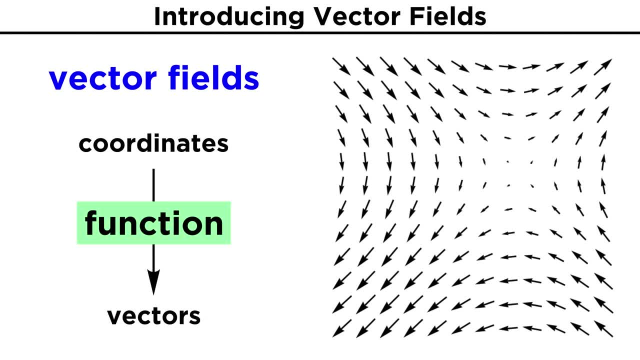 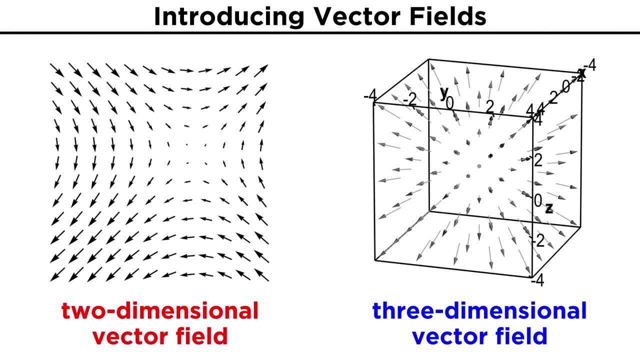 coordinates and give back vectors. These vector fields will end up having vectors assigned to every point throughout the coordinate system, as shown here. Of course, we are not limited to just two dimensions. Vector fields can exist in any number of vectors. Vector fields can have a number of dimensions, and an example of a three-dimensional field: 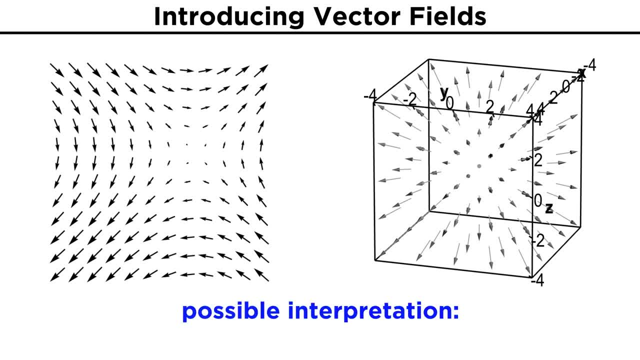 is shown here. These vector fields can have a variety of practical interpretations, such as a force being exerted through space or as the representation of motion. But for now we will just focus on the general concept of a vector field and cover some basics. 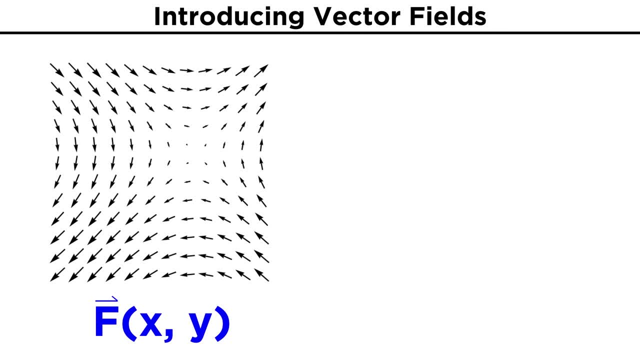 As we mentioned, these vector fields can be thought of as functions that take in coordinates. They can be thought of as functions f of x and y, where the function has vector components that depend on the coordinates x and y. The most general way we could express this is: f of x- y equals p of x, y, i plus q of x. 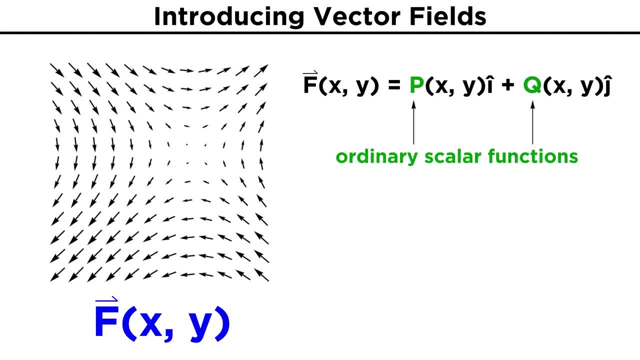 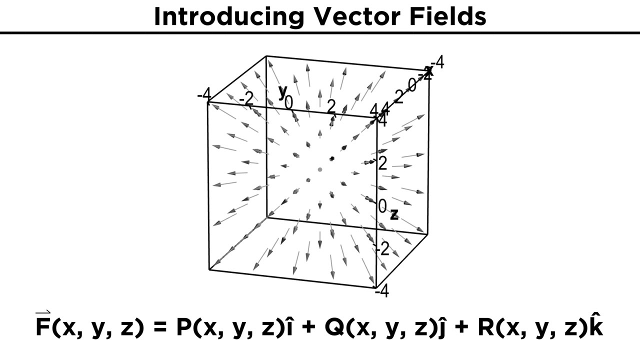 y, j, where p and q are ordinary scalar functions that will depend on the coordinates x and y. These, sometimes called scalar fields determine the components of the vectors at each point in the coordinate system In three dimensions. our vector field could look like this: 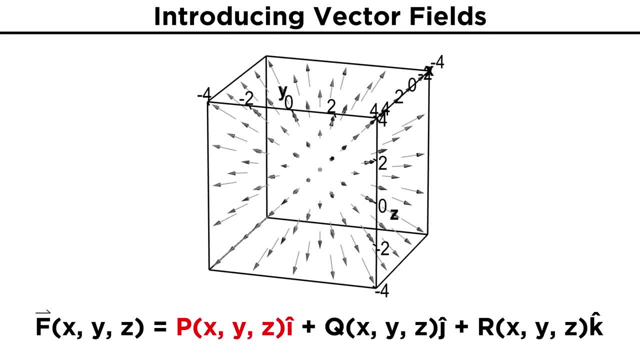 F of x y z equals p of x y z i plus q of x y z j, plus r of x y z k. For a quick example, consider the vector field. f of x- y equals p of x y z i plus q of x- y. 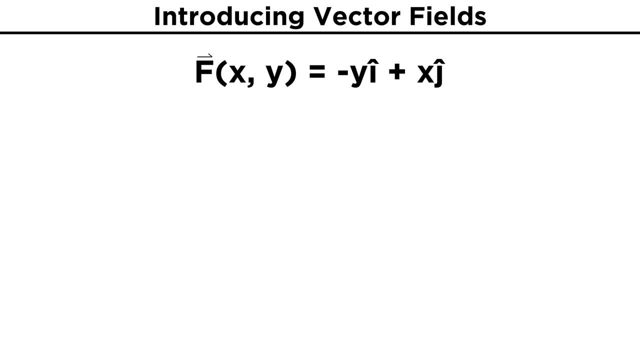 z, j plus r of x, y, z, k. To get an idea of how this vector field looks, let's plug in a few coordinates and plot our resultant vectors. We will take a few simple coordinates of the form and plug them into the vector field. 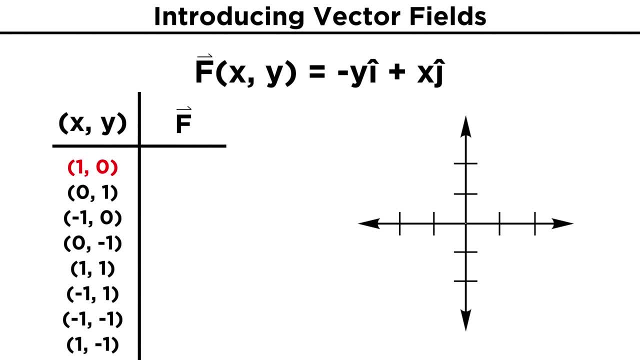 To start, consider Here: x equals one and y equals zero. so we get back the vector. We will now plot this vector originating from the coordinate we plugged in. We can quickly go through several more points and plot the resulting vectors as we go. 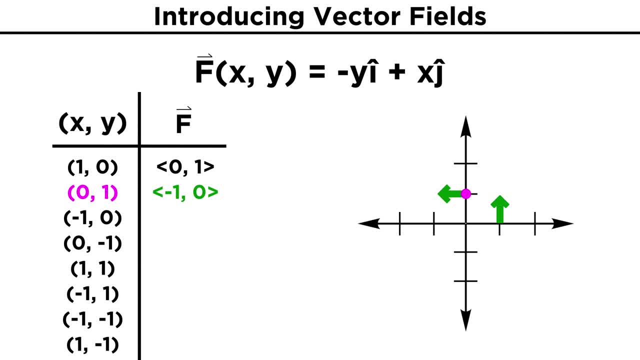 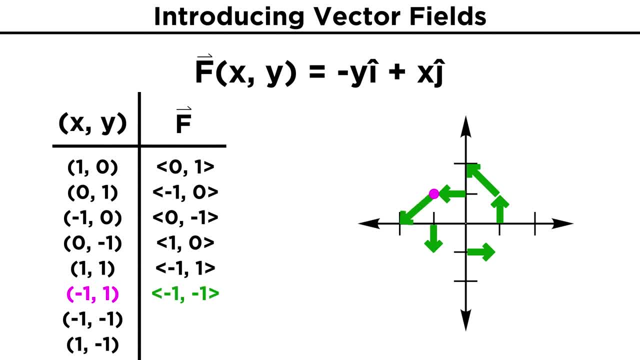 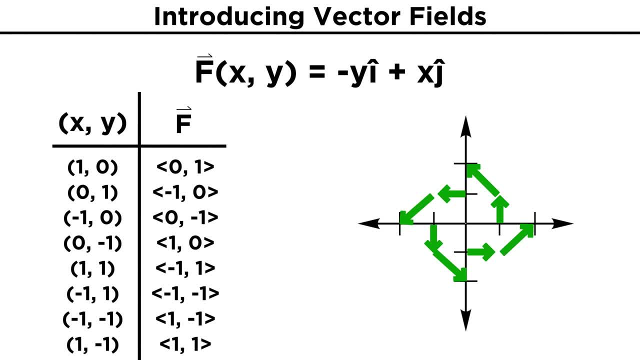 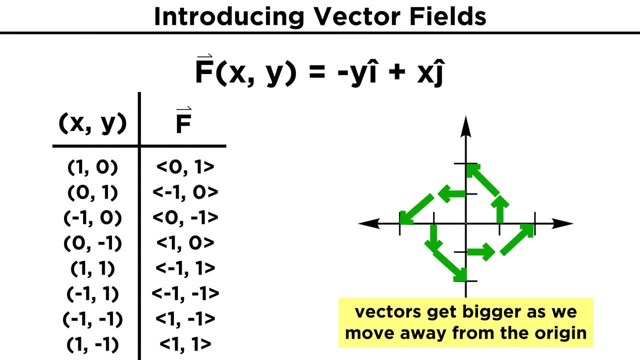 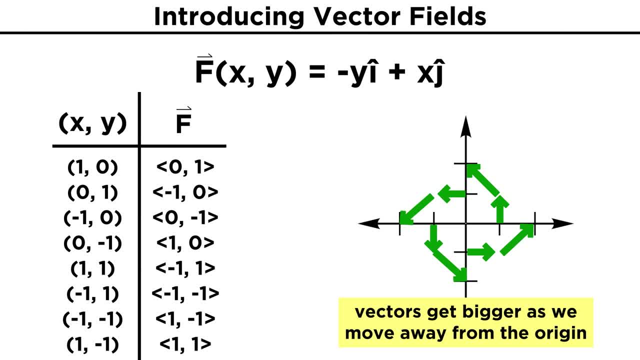 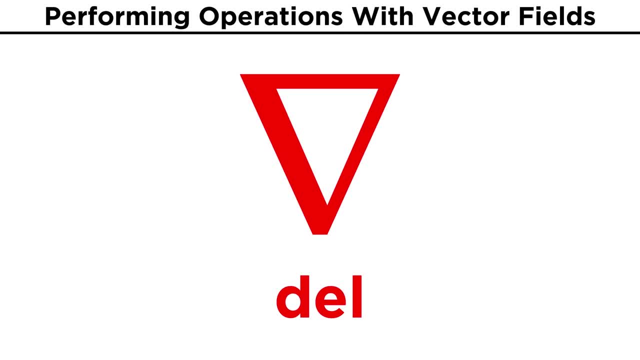 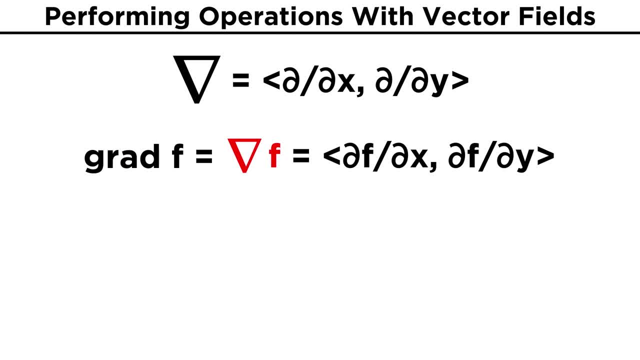 The gradient of some function f, del f is itself a vector field with components being the partial derivatives of the function. so df, dx, df, dy, To get more specific, if we have a vector field f and it can be written as the gradient, 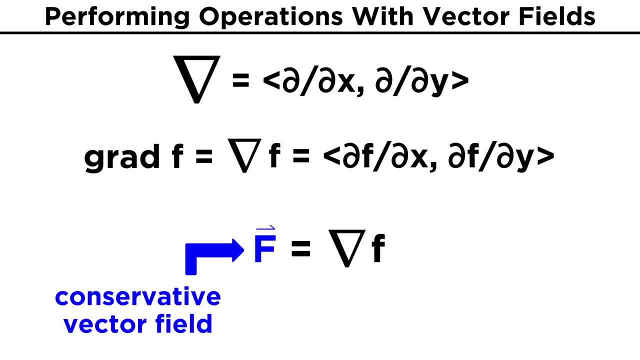 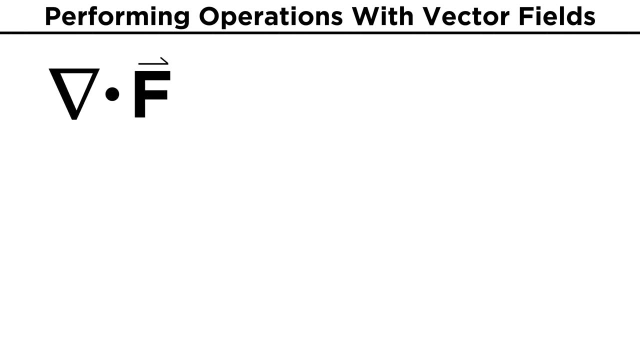 of a function f. the vector field is called a conservative vector field and the function f is called a potential function for the vector field f. There are two more uses for the del operator with vector fields, and these involve the vector dot product and cross product. 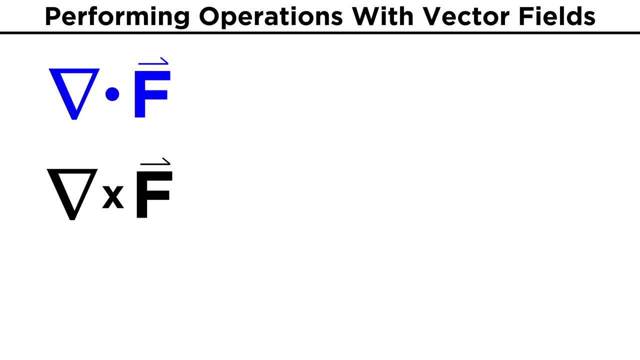 We can take the del operator and dot it into a vector field f. This is referred to as the divergence function. Similarly, we can take del cross f, and this is referred to as the curl of f. Let's take a closer look at what these expressions are. 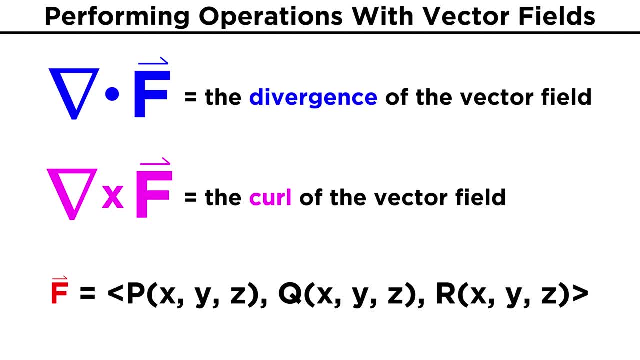 Recall that we can write a vector field, f, in the form pxyz, qxyz, rxyz. so for now we'll just focus on three dimensions, while p, q and r will be ordinary scalar functions that depend on f. While we can take the divergence in any number of dimensions, the curl can only be taken. 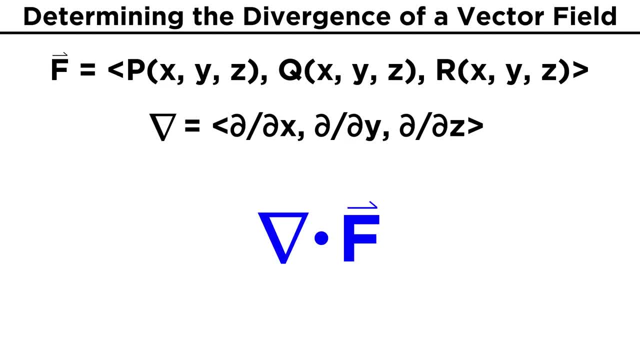 in three dimensions. First let's look at the divergence del dot f. Recalling from a previous tutorial how the dot product works, we will simply find the product of the corresponding elements of the vectors and then add those up. so del dot. 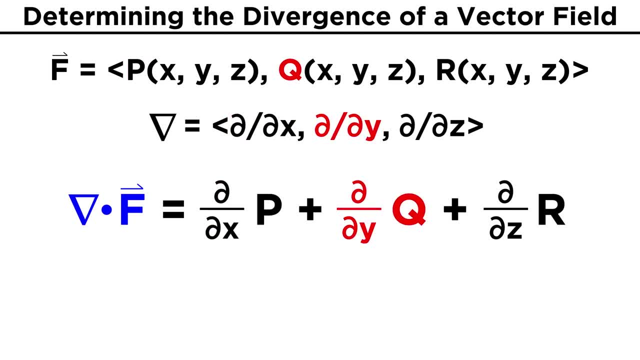 f ends up being f, This will give us ddx, p plus ddy, q plus ddz r, which means we take the partial derivative of p with respect to x, plus the partial derivative of q with respect to y, plus the partial derivative. 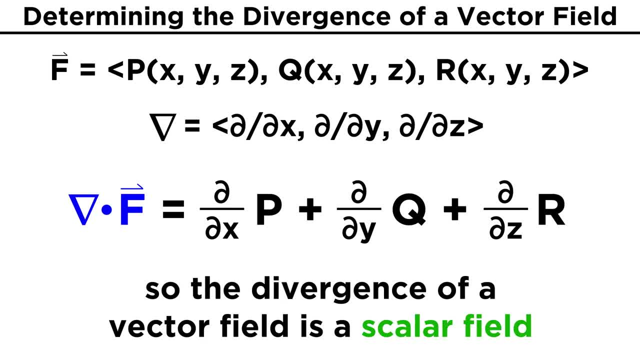 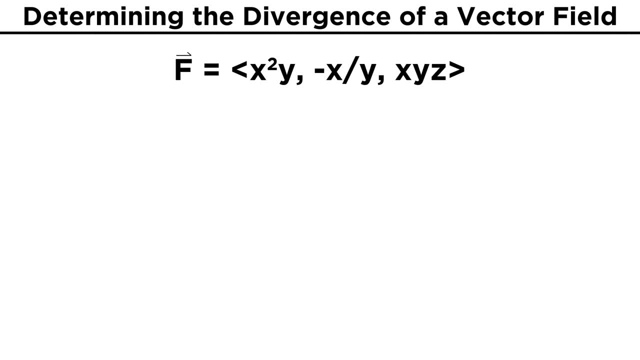 of r with respect to z. So the divergence of a vector field will no longer be a vector field, rather it will be a scalar field. Consider the vector field: f equals q. Let's take a look at the divergence. equals x squared y, negative, x over y, xyz. To find the divergence, we will take del dot. 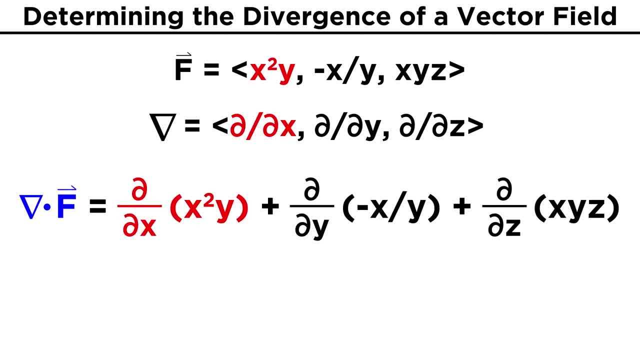 this expression, which gives ddx- x squared, y plus ddy- negative x over y plus ddz xyz. All of these derivatives follow the power rule that we already know, so we end up with 3xy plus x over y squared plus xy, which simplifies to 3xy plus x over y squared. 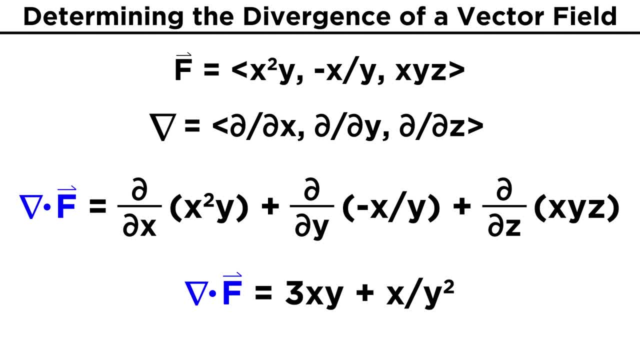 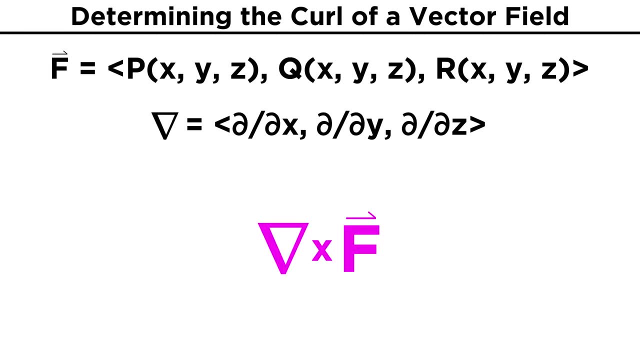 We will get more into the application of divergence in a future tutorial, but for now, you can think of it as a measure of how much of the vector field is going out of some point Now. Next, let's go over the curl. As we mentioned, the curl will be the cross product between: 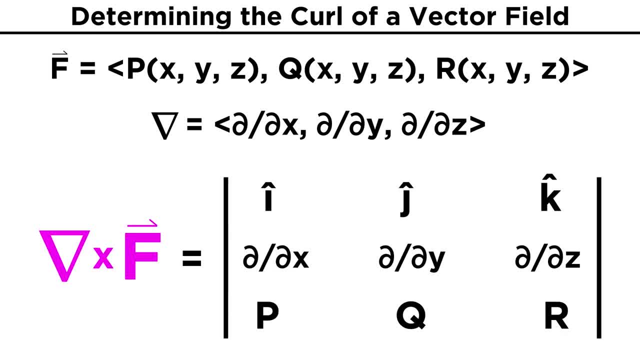 del and a vector field F. Remembering how the cross product works from a previous tutorial, we set up a matrix with i, j and k on the top row, the elements of del on the second row and the elements of F on the last row. Let's once again consider the vector field. 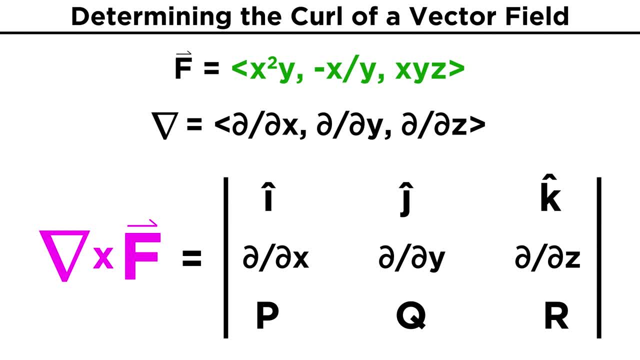 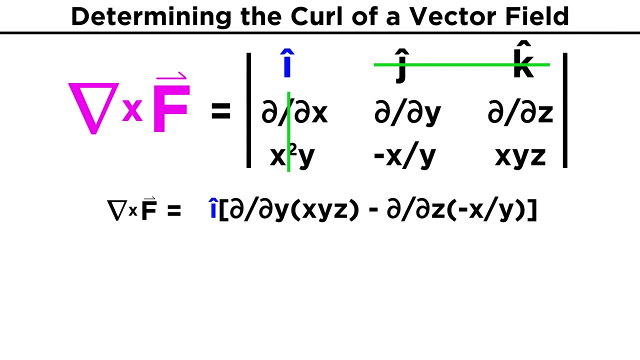 F equals x squared y negative X over Y XYZ. To find the curl we will take the determinant of the matrix IJK, DDX, DDY, DDZ, X squared Y, negative X over Y XYZ. From the determinant we get, I times the quantity DDY XYZ minus DDZ negative X over Y minus. 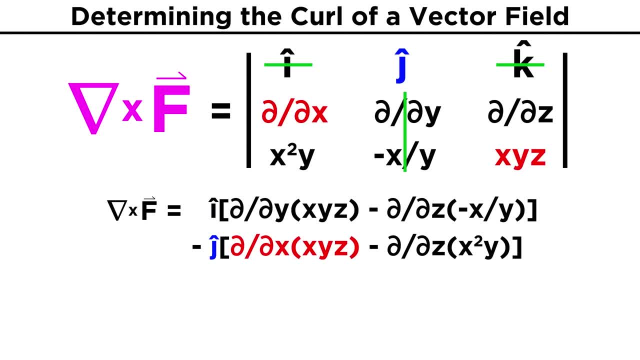 J times the quantity DDX XYZ minus DDZ X squared Y, plus K times the quantity DDX negative X over Y minus DDY X squared Y. Now we take all these derivatives For the first term, this Y becomes one, so we get XZ and this expression has no variable. 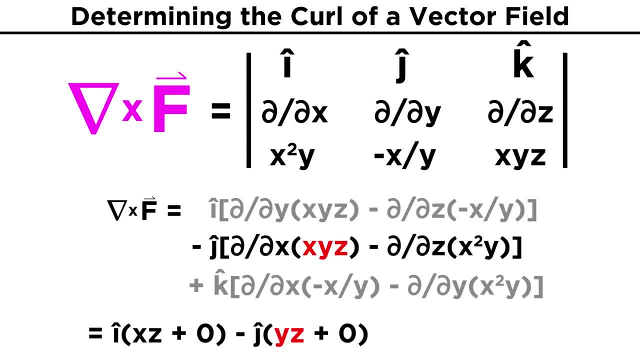 so it becomes zero. For the second term, this X becomes one, so we get YZ. and again here there is no Z, so this becomes zero. For the third term, this X becomes one, leaving us with negative one over Y, and this Y becomes. 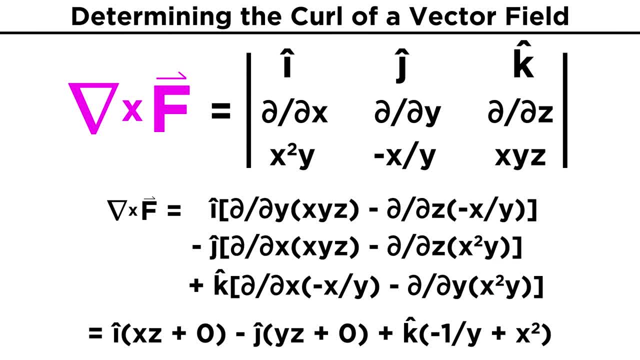 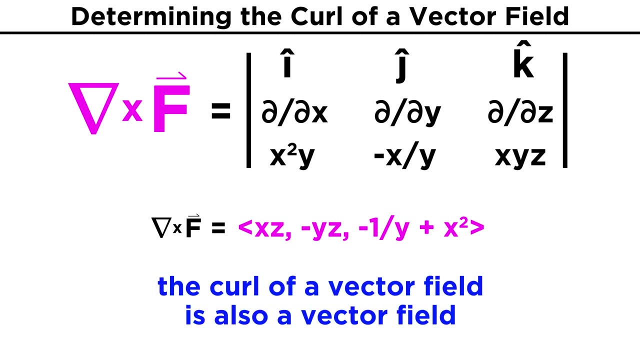 one Simplifying, we get XZI minus YZJ plus negative, one over Y plus X squared, K. or in vector form: XZ negative, YZ negative, one over Y plus X squared. This is the curl of our vector field. 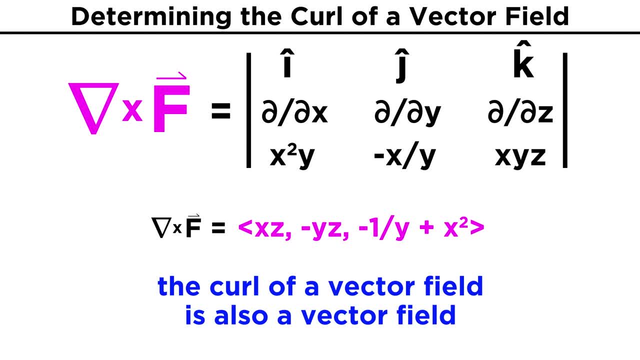 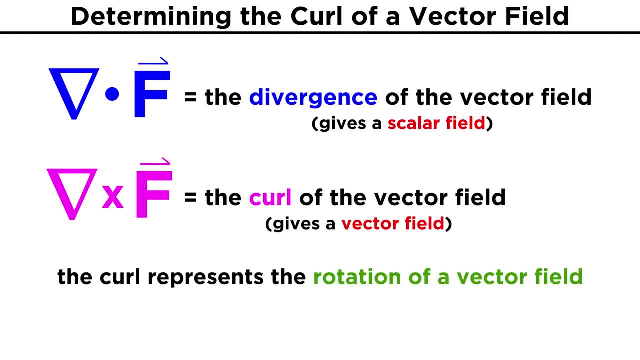 Notice that the result is also a vector field. So while the divergence is a vector field, the curl is also a vector field. The divergence gives a scalar field. the curl gives a vector field. The curl represents the rotation of a vector field F, the direction of the curl being 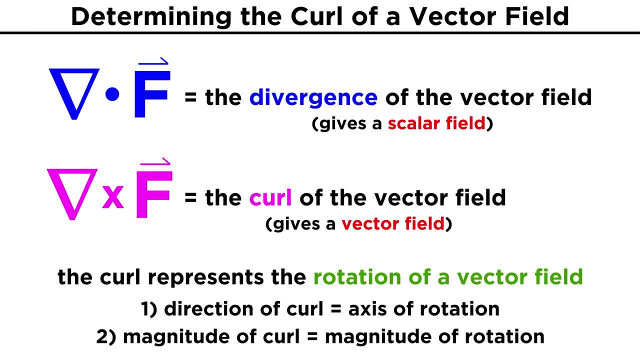 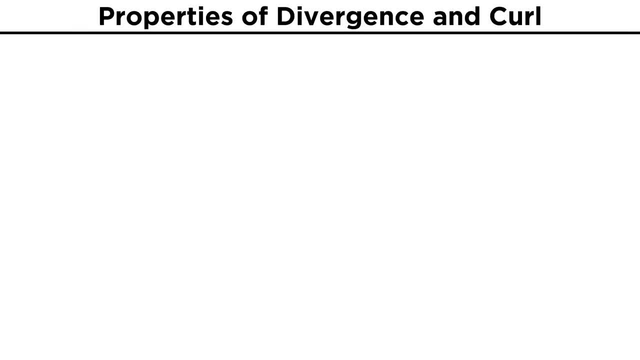 the axis of rotation and the magnitude of the curl being the magnitude of rotation. Before we wrap up, let's mention some interesting properties of divergence and curl. First off, for a function that has continuous second order partial derivatives, conservatives, the curl of its gradient is always the zero vector. 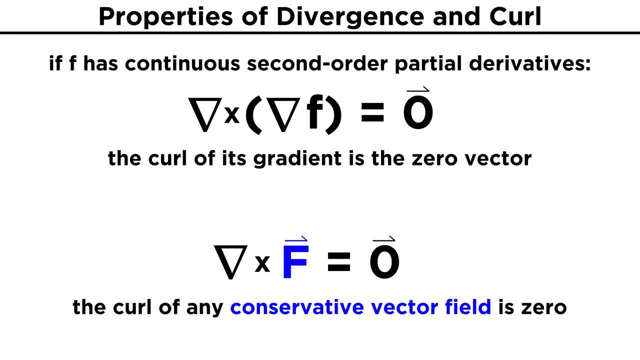 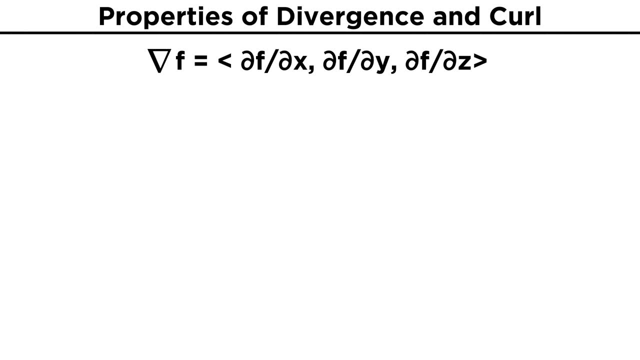 This means that the curl of any conservative vector field is zero, because being conservative means the field can be written as the gradient of some function. We can go ahead and show this by writing the gradient as and taking the curl. To do this, we set up the matrix shown here and take the determinant. 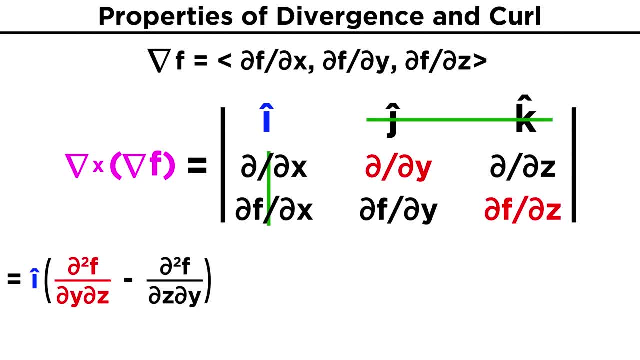 We end up getting i times d squared f dy dz. minus d squared f dz dy minus j times d squared f dx dz. minus d squared f dz dx plus k times d squared f dx dy minus d squared f dy dx. 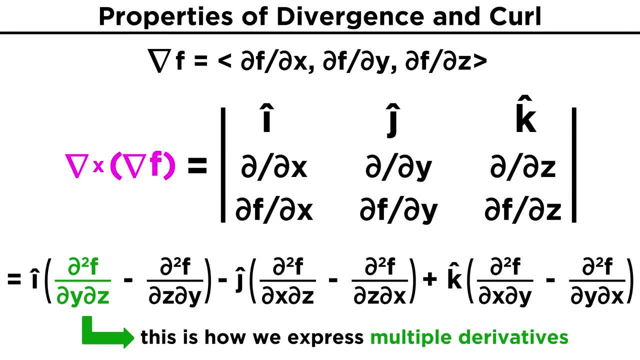 This notation is how we express taking multiple derivatives of the function f, with the order of differentiation being the variables on the denominator from right to left. If we took the derivative with respect to the same variable twice, say x, it would be expressed as: d squared f, dx squared. 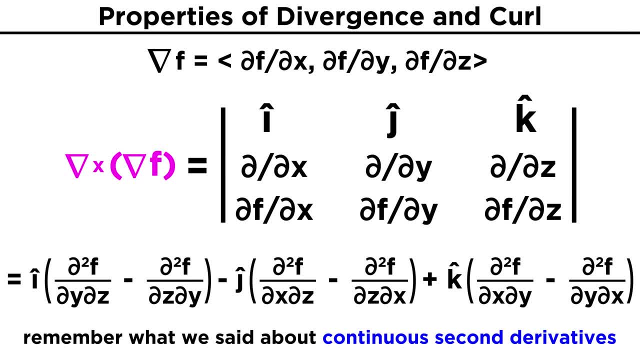 Now here's where we need the continuous second derivative to come into play. If these derivatives are the same, then the derivative is the same. If these derivatives are all continuous, that means the order in which we take derivatives does not matter, meaning that d squared f dy, dz is the same as d squared f dz, dy and. 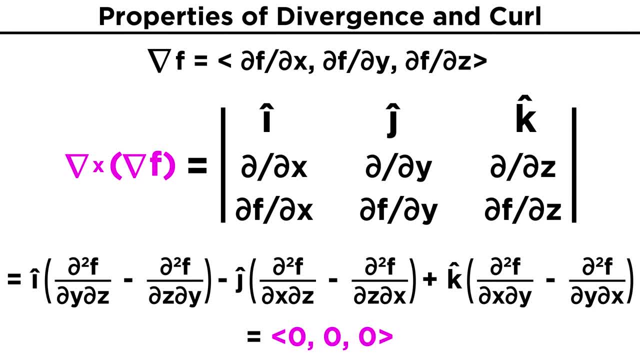 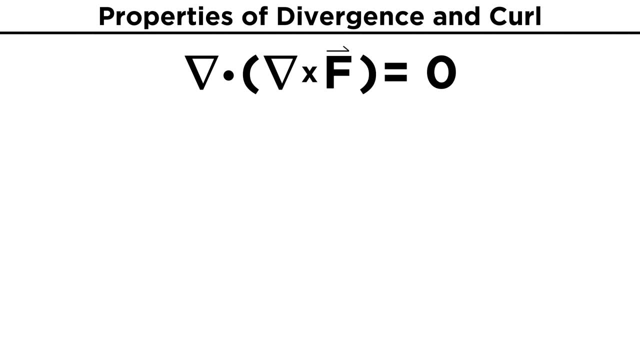 so on. So all of these terms cancel and we are left with a vector that has a zero for all its components. This is the zero vector and we have proved this property. Another property is that if the components of f have continuous second order, partial. 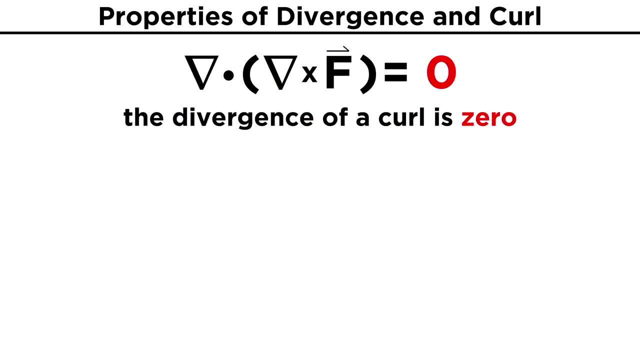 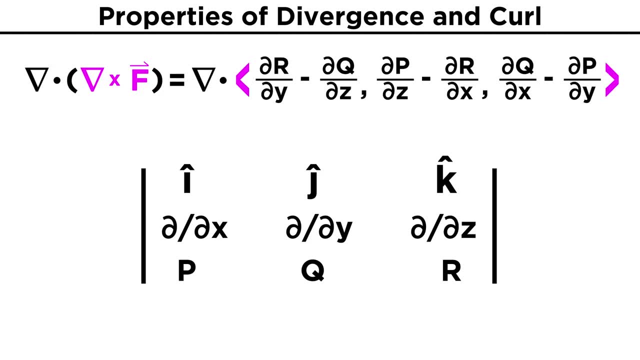 derivatives, then the divergence of a curl is always zero. We can prove this as well Jumping ahead and writing out the components of the curl. we get del cross f being equal to dr dy minus dq dz, dp dz minus dr dx, dq dx minus dp dy. 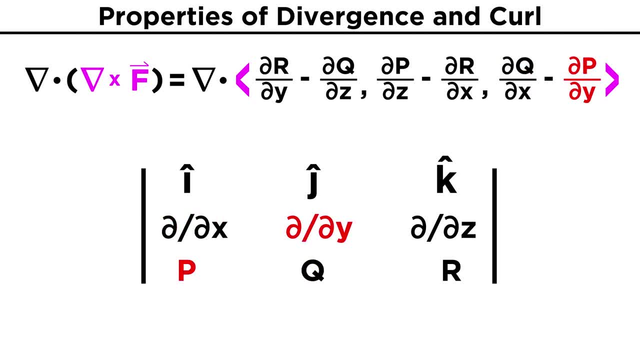 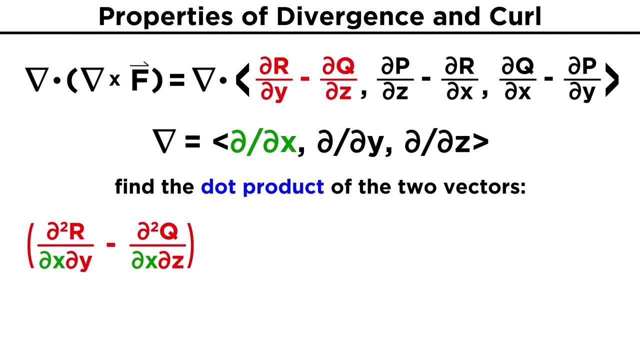 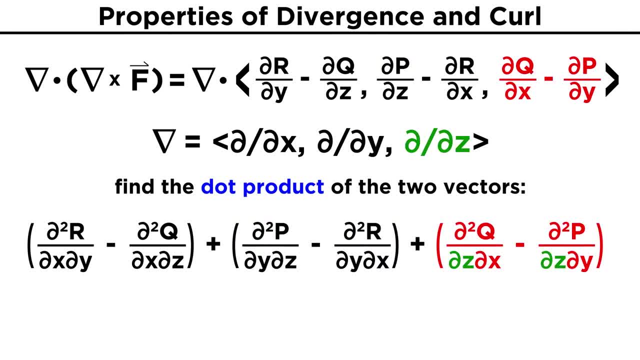 of the second with respect to y, plus the derivative of the third with respect to z. This gives us d squared r. dx. dy minus d squared q. dx. dz plus d squared p. dy. dz minus d squared r. dy. dx plus d squared q. dz. dx minus d squared. 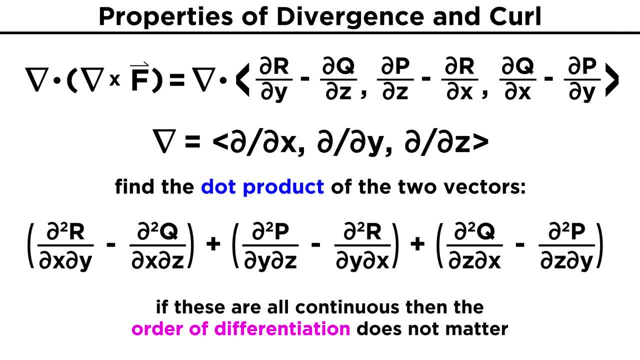 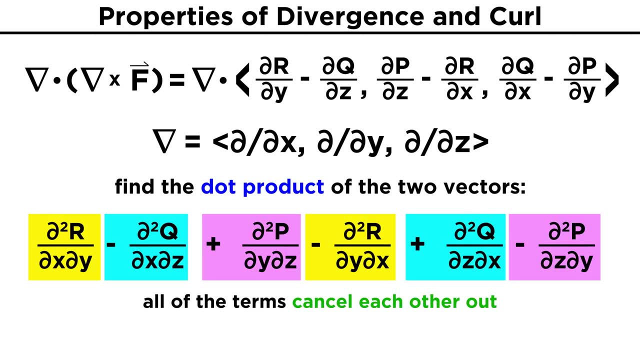 p, dz, dy. Once again, if these are all continuous, the order of differentiation does not matter and since this is all just one long series of terms being added and subtracted anyway, we can find the corresponding terms and get them all to cancel, giving us zero and therefore. 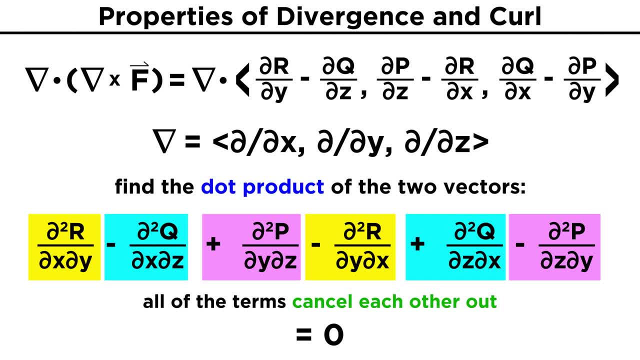 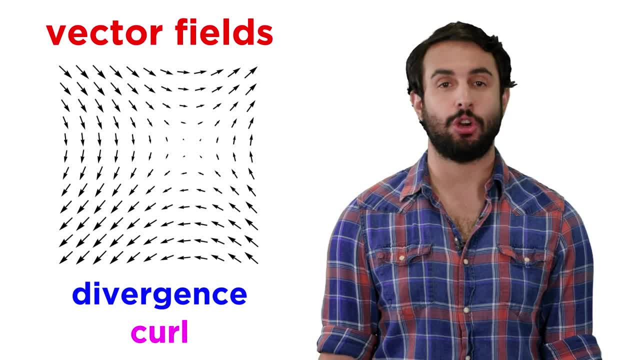 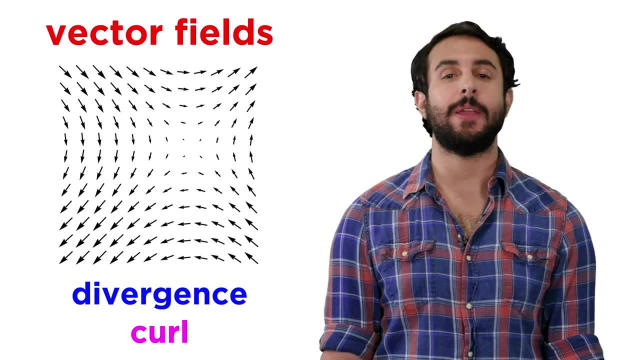 verifying the property. Vector fields are a very useful concept, and being able to take the divergence and curl of these fields allows for a surprisingly wide variety of calculations. There are several important theorems that utilize these operations, so let's check out some of those next.